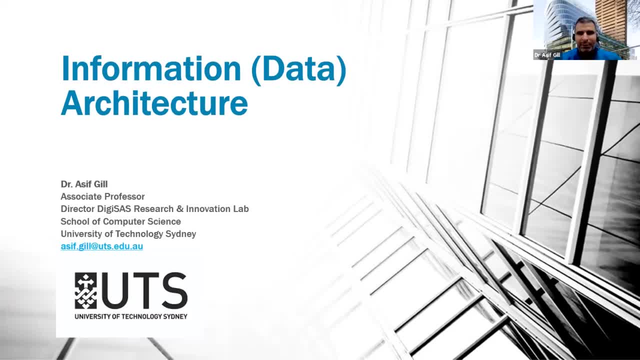 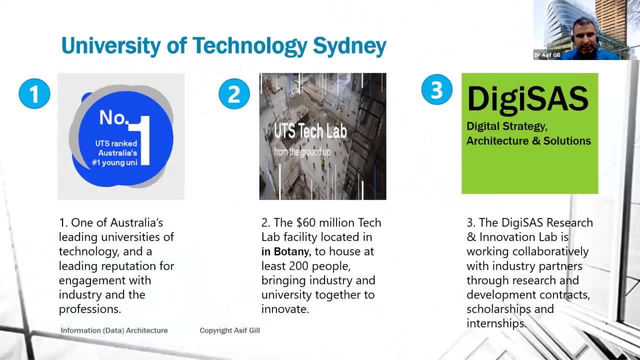 because I believe data is an implicit part of information. So when we are discussing information, we are implicitly discussing data as a part of it. So that's the mindset behind it. So, as Andrew said, I work at UTS. I lead DG SAS Lab, which focus on digital strategy architecture and 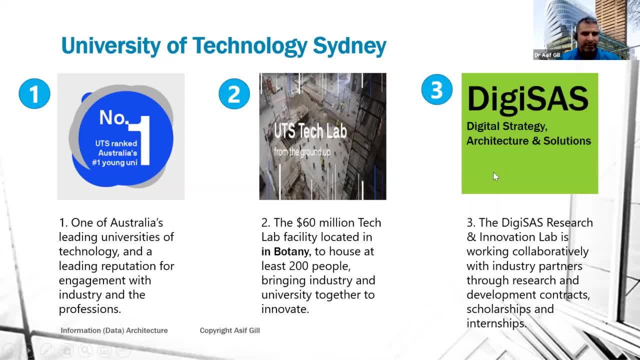 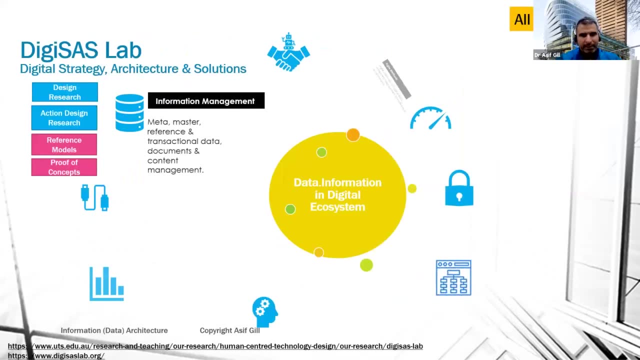 solutions And as a part of that, UTS is that we are number one university in terms of tech at least, And my whole work around is the data and, in particular, data strategy, architecture and solution in the digital environment. Just giving you some background: what kind of work. 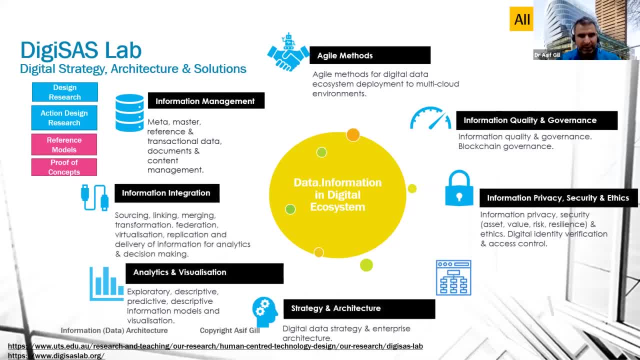 involved when we talk about digital data or architecture. So when we are architecting data or information, we are looking at really data and information in the ecosystem context, which is a digital ecosystem context where it is by default. we assume data will travel. 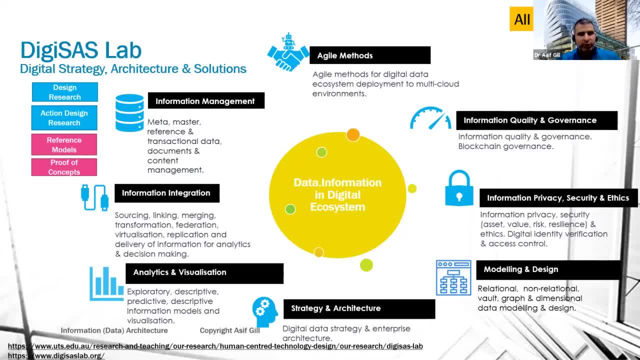 beyond the boundary of a single enterprise, It will be shared. So that's different from the when you design architecture of the data or information within the single environment or single enterprise boundary. So as soon as leaves the boundary it quite gets complicated. So in 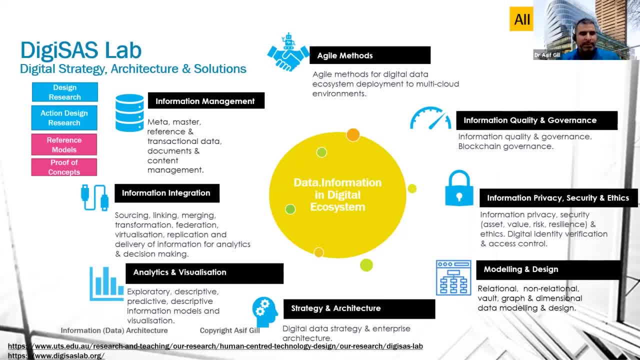 our lab we study information and data, which is a part of the information science discipline. We look at that agile matters for handling data, And then we're looking at the information quality and governance. We also look at the information privacy security ethics in this lab We 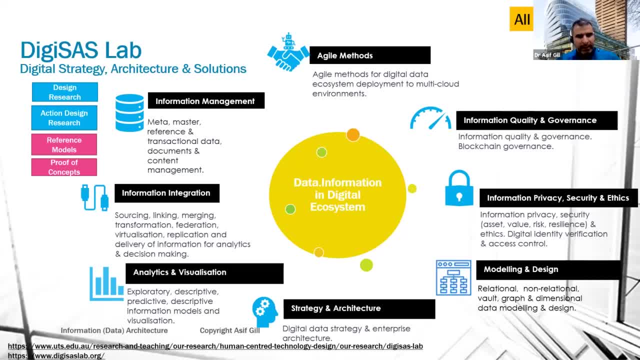 also look at information modeling and design part of the data, information. Also look at the strategy and architecture of the data and information as well, which is a today's topic is actually, And we also look at the visualization analytics of the data, information and integration. 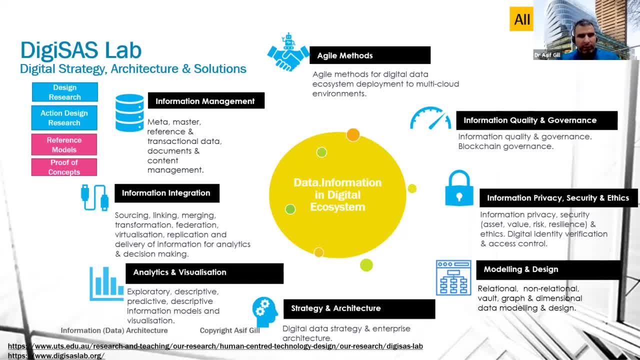 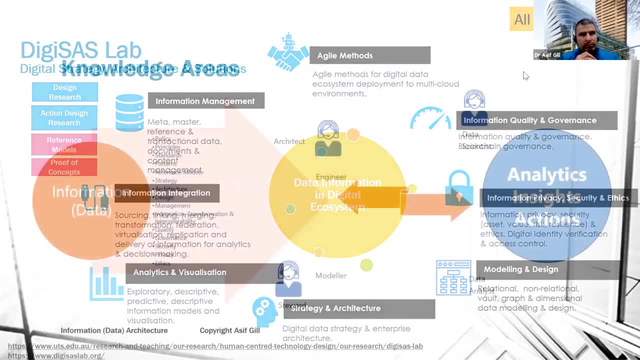 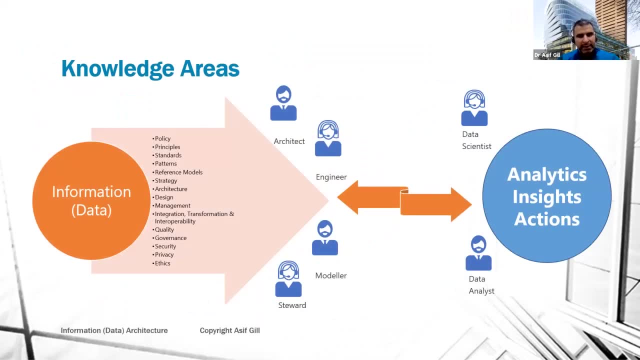 and overall information management. So this is a kind of all things around information or data we deal in in this lab. So the question is that I think we have a full two day workshop is planned as a part of the data modeling zone conference, which is 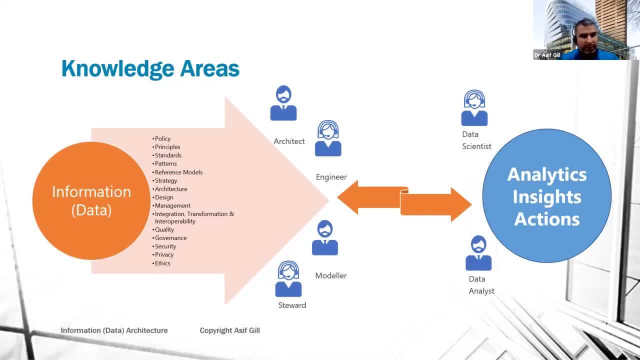 a schedule towards the end of June, As you probably some of you have already seen that, probably maybe on the web or LinkedIn, So I'm just going to highlight a few things in today's presentation where the detail would be in that two day coach, It's about the knowledge area. When we look at 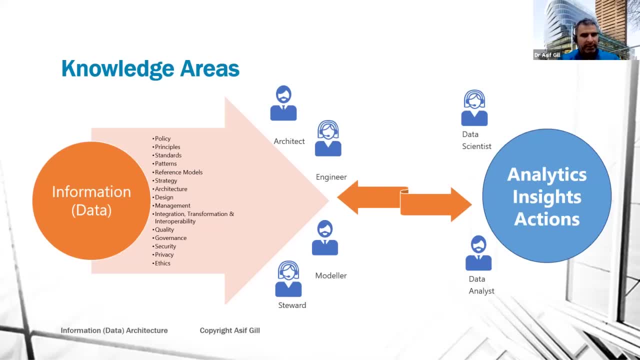 that data landscape, information on data, what are the different aspects of the data landscape, What are the different roles involved and where the architect would fit? And you can see that when we're looking at the information on data, we're dealing with a lot of things. Let's say we're 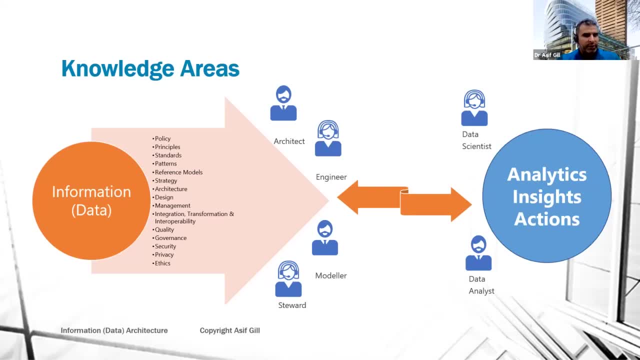 looking at the policy principles, standards, data or information patterns, reference model, strategy and architecture, which is today's topic, And then information design, which is different from actually the architecture. a lot of people confuse the information design because 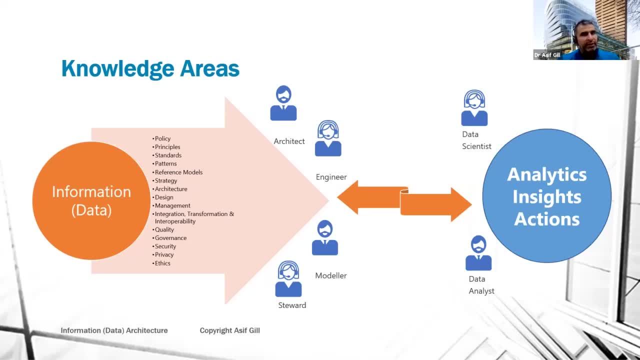 initially information architecture or data architecture emerged as a information design in 70s or 80s And then later on it became more strategic in nature and more business oriented, And that's what we call information architecture is more towards that design could be a little bit more. 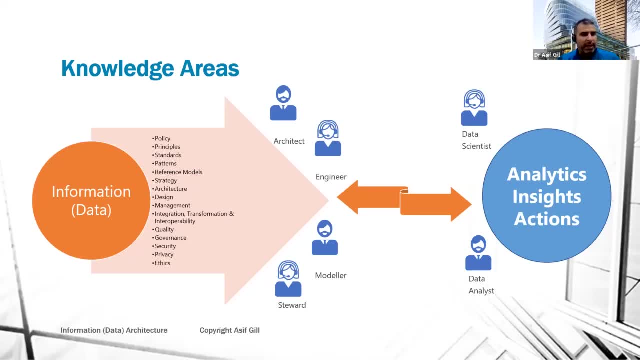 low level modeling of the data or information and then how we manage that, integrate transformation sharing into probability and all those things. we look at that. So different roles attached to that is not a one person's job. Some of the roles are there If on the data side, 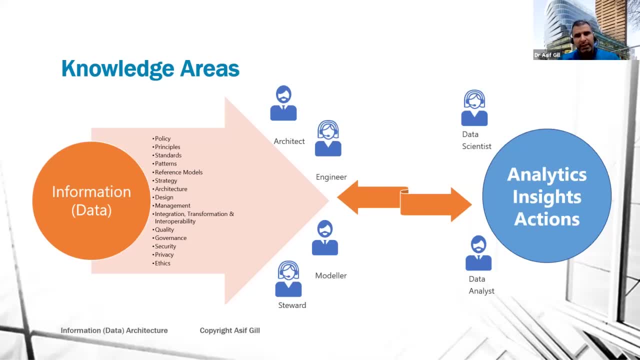 we have architects, data engineers, data modeler, data stewards and, on the other side, your data scientists and data analysts, who actually consume or use the data for analytics, insights and actions. So really is before we get to the stage of analytics and insight and action. 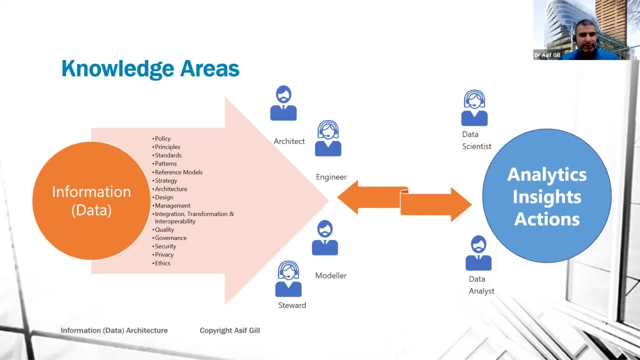 we really need to be able to understand our data environment and being able to design or architect that data environment So that the data, the data environment or data architecture can manage that is fit for purpose. So the analytics, so a lot of work happens here. before it jumps over here, I would say that rule. 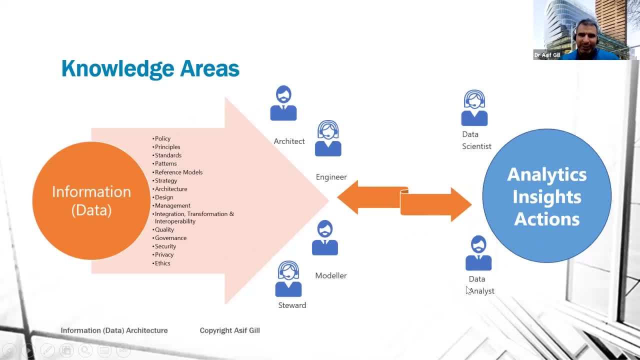 of 80, 20- 80% work is done around the area where 20% work is done over there. So that's where the architect role really becomes really important. They're looking at the overarching corporate data or enterprise data and linking it with the strategy, and then downstream data or information. 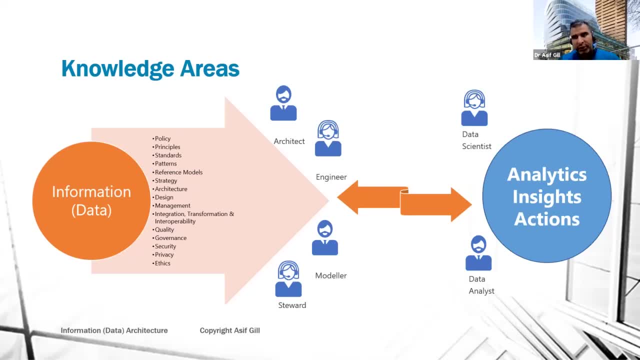 roadmaps and solutions as well. So really, architecture is a kind of a meat in a sandwich as a role point of view And in my experience of last 20 years or so, I think we have a shortage of data, information architects in industry and we really need those people to come up and being able to train and 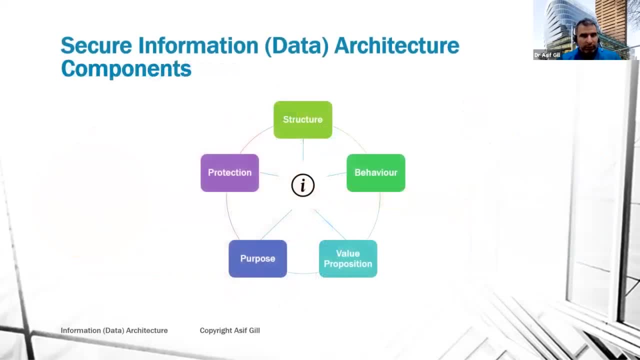 gain skills in that. Now, what is in the architecture itself? when we're looking at that, I call that secure information data architecture component. So essentially the information security sometimes is considered kind of a separate from information architecture, which is okay, But really the both disciplines of information security and information architecture 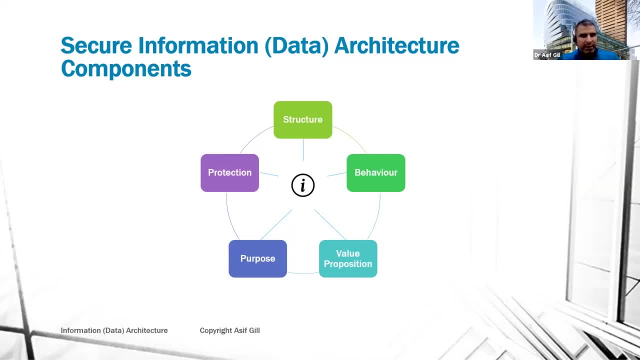 they need to work together, they need to be integrated together. So that's where it is secure information data architecture. we call it because security or protection needs to be part of the design of the architecture, in embedded in the old layer of the architecture. 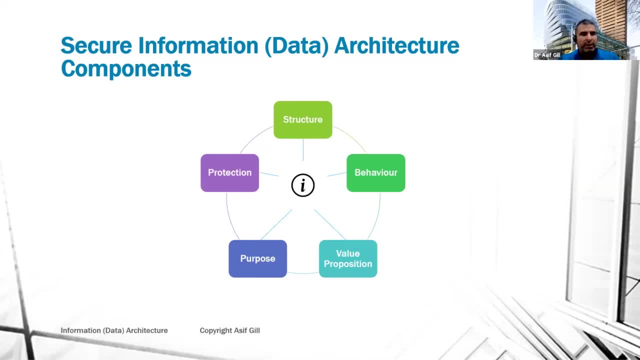 So that's where protection- secure- is really important. But if you look at the very high level, what are the? when we talk about architecture of the data or information, what are the really the components we need to deal with it? So there are five very high level components we're dealing. 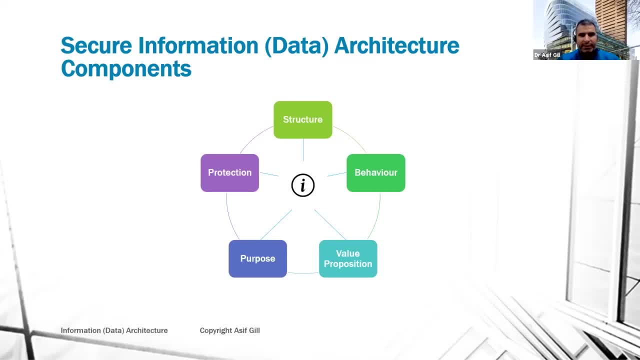 when we're looking at the secure information or data architecture. One is: architecture is about describing understanding the enterprise information or data structure, which includes the database here, the really major aspects of the database, as well as home page variables, that your website and its object provides. That's actually why we're using data structure is 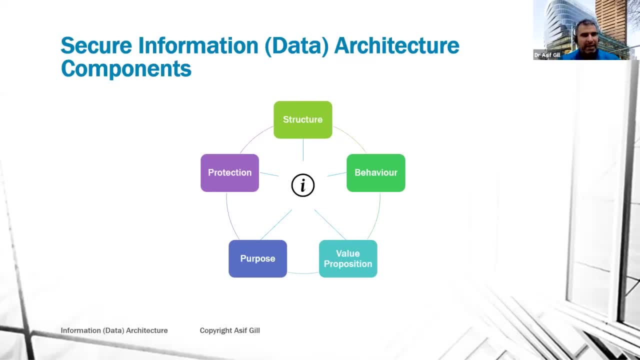 because we are using the data structure to enjoy open space, which really is that the cells may одинate with individual environments. that examples not all of the fields on your site, And then we're looking at that structure has further some behavior as well, like any architecture, like the. 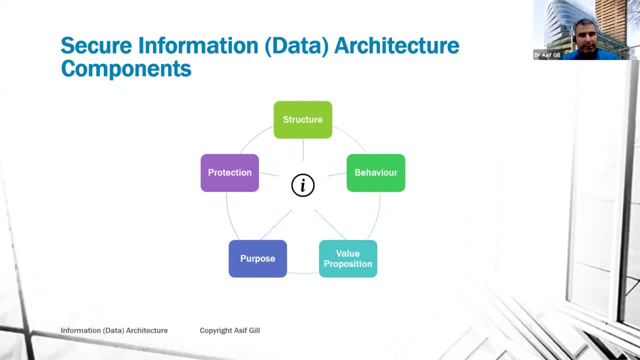 building example you can take that building has a behavior or use case. so information as a use case of behavior or its process. so here we're looking at the structure which which is being processed by the certain behaviors or processes or use, the process which in all your information management information. 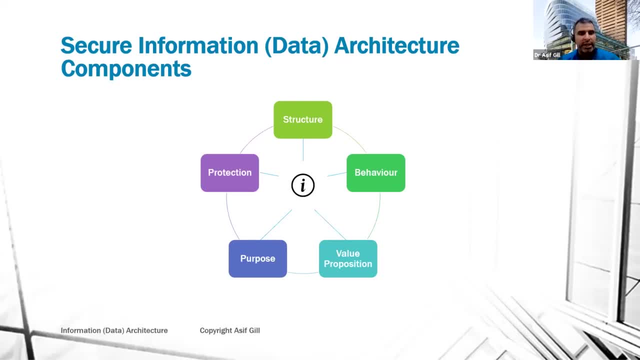 integration, classification, sharing, storage, you name it. so we really need to look at the information behavior across the enterprise as well, and when we talk about the information ecosystem architecture, we're looking at beyond the boundary of the enterprise. so behavior or process, the process or structure, and they produce some value proposition where we're looking at really what, what, 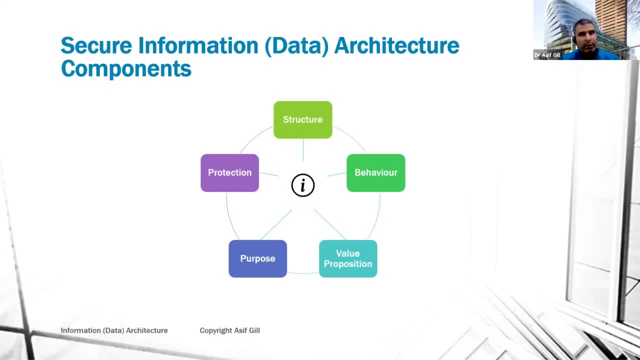 are the different information or data, products or services being consumed, produced by the enterprise with operating in the ecosystem. so really, we looking at what is the value proposition. yes, we understand the information structure, we understand its behavior, but what is really a value for us? why are we doing that? and that's where we're. 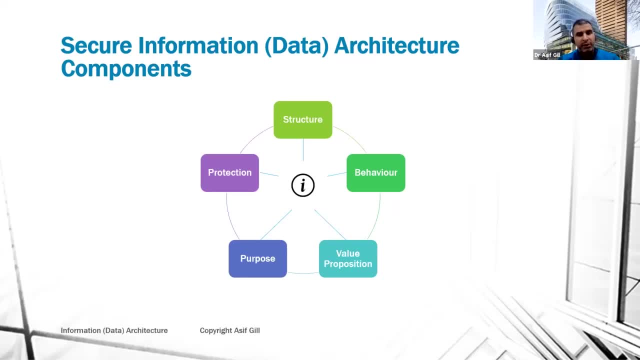 looking at the value proposition, information or data, products or services we need to, which we need to design- and that's also described as a part of the architecture as well- and most important thing is that there's certain purpose behind that regarding the structure, behavior and value proposition. all have attached purpose, which we call information. 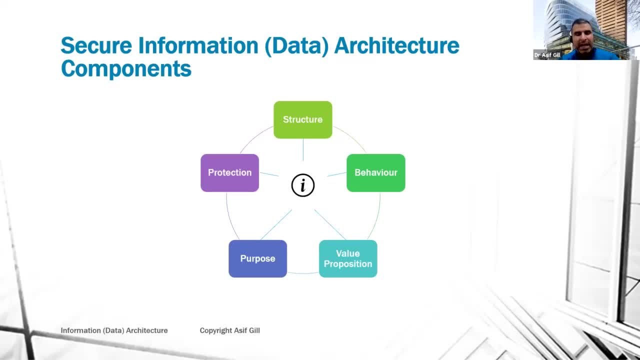 purpose and that's very, really, information architecture is linking back to the information or data strategy, and information data strategy is a part of the bigger IT strategy or a business strategy, wherever it sits in your own organizations. and finally, we also need to look at the protection of the 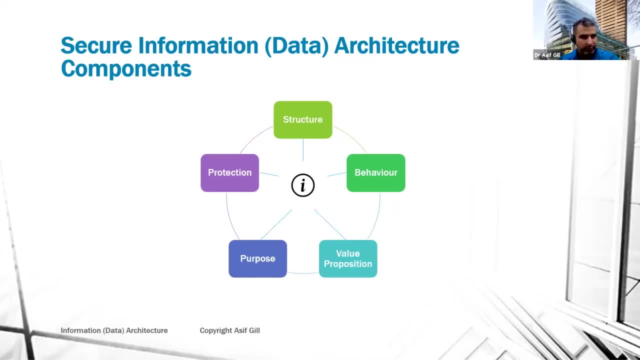 structure, behavior and the products as well, say. we're looking at the overarching protection, which involves security, privacy, ethics and all these things around the safeguarding of the data or information from risk, vulnerabilities and threats. so this is all about very much the five components of any information data architecture at 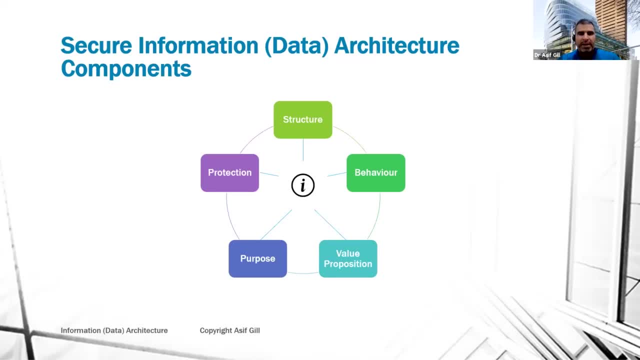 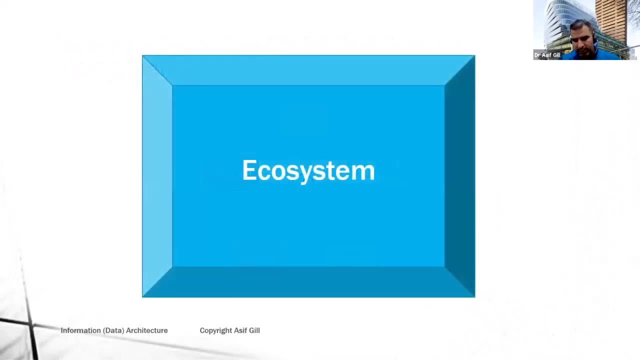 the very high level, and your architects in your organization should be able to process the data and being able to design the data architecture using these five type of components. in the course we will discuss in detail how we go about it, but I'm just introducing you in today's 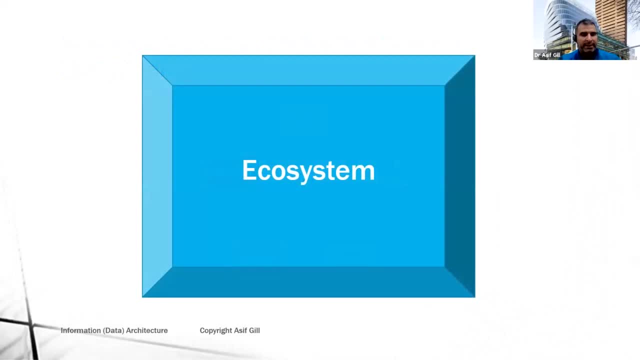 webinar webinar- what we really mean by data architecture. a lot of people have a lot of confusions around that. another thing: I mentioned that data sharing is by default in the current modern world of digitally connected world. so we have ecosystem perspective. there are different day actors, ecosystem actors. 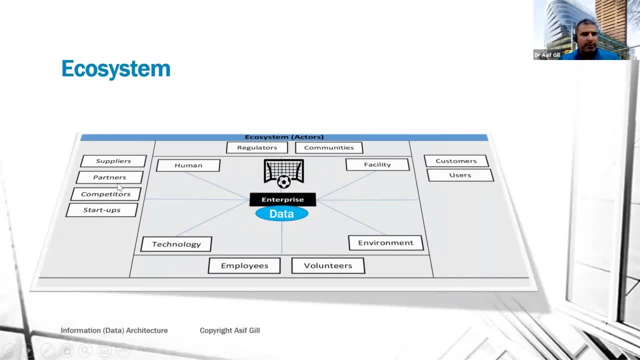 including enterprise says enterprise data here. like suppliers, partner, competitors, employees, volunteer customers, users, other people, communities, regulators- all they actually interact with your data. so we need to consider data being a part, or information being a part, of the whole ecosystem when we design the architecture. we can't just think of the data or assume the data or 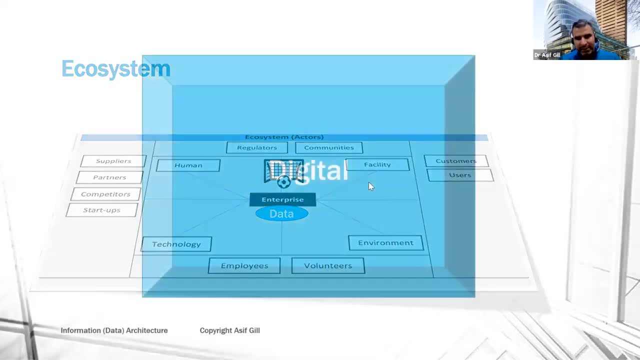 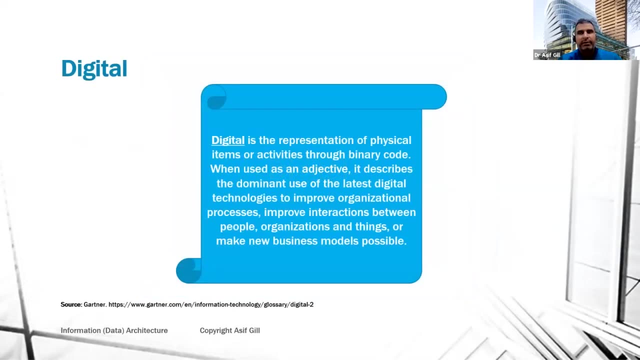 information will stay in the boundary of the enterprise. so that's a really mindset. second thing is that increasingly becoming digitized and enterprise architecture and within that, information architecture and data architecture, is becoming so critical because we being digital or digitalized is becoming so critical because we being digital or digitalized 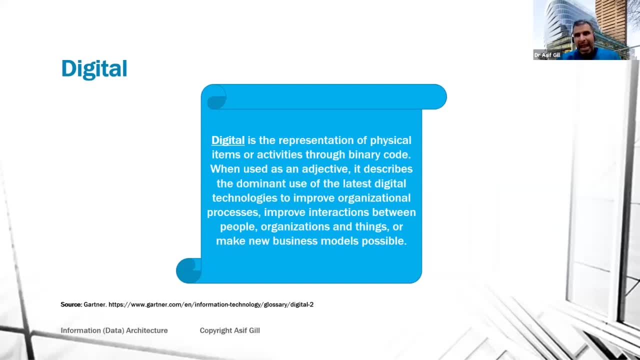 generation, generating a huge amount of data, if you do not handle the data or information as a strategic asset, that's going to be a really challenge for us and that's where we need to have a data information strategy and the architecture to realize that strategy of the data, information and digital asset. 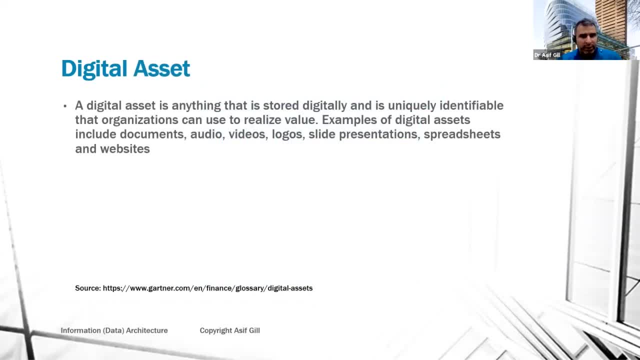 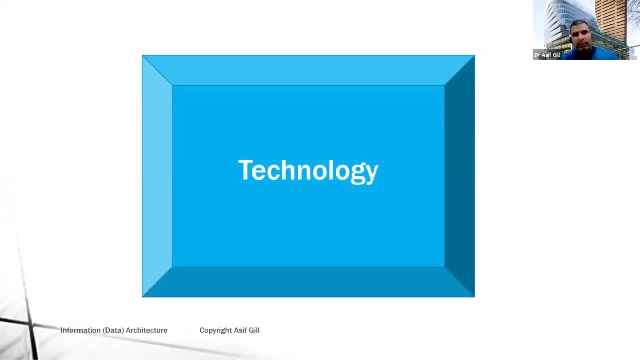 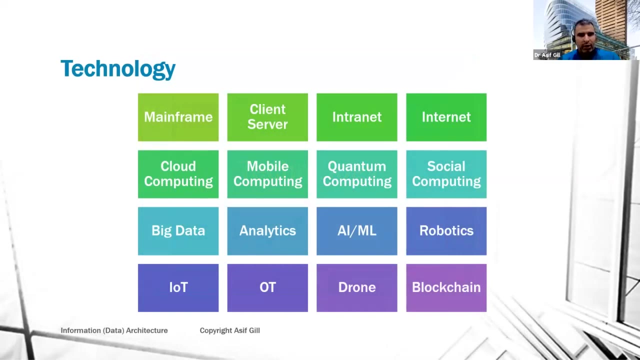 in terms of our information or data, all those products which we build as a part of our architecture. that's really looking at that and once we look at that, what information as digital asset we have. we also look at a technology which actually enables us to handle or process or store or integrate or share that data. 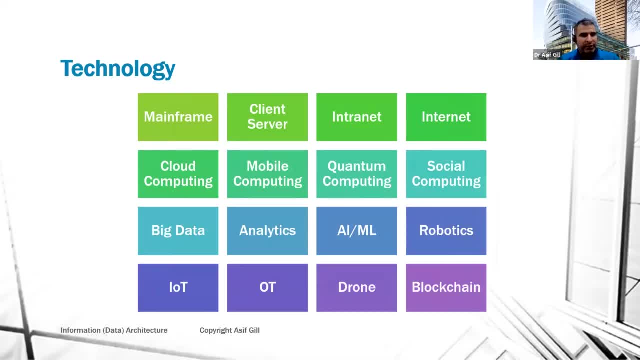 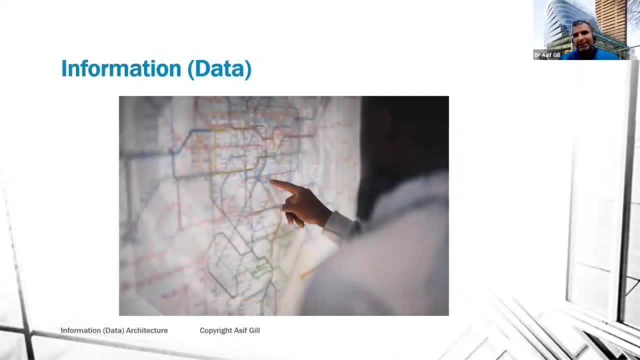 or information. that's also part of our architecture as well. and then you name it, and the most important in the architecture is that actually the information and data and information on data I call a information- is a collection of data elements, so each information element, one element, could have a. 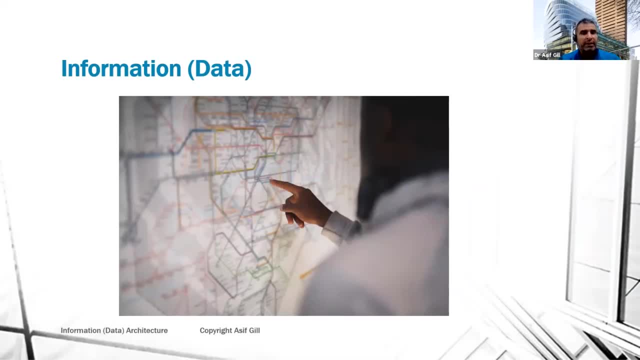 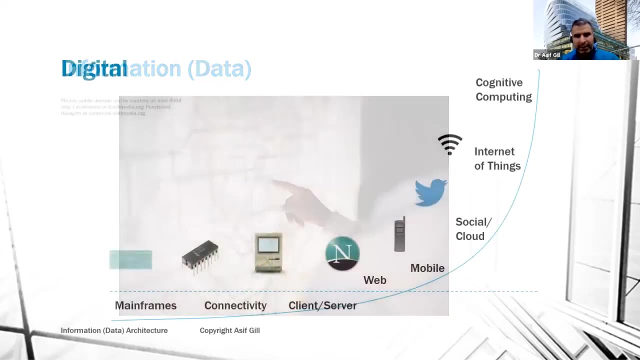 multiple data which are linked together and whose life cycle is managed as a group within the information element. so that's how information is defined. data is an implicit part of information and it's linked, as you can see the map as well here. as we increasingly digitize, more information, data is being produced and 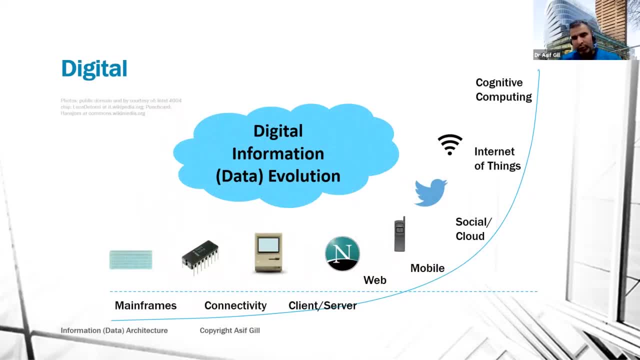 more challenges we have if we are don't have the architecture practice from information data part of we set it up internally. that's really we calling for a disaster. we'll be developing the hawk applications, analytics and algorithm and we will be sub optimizing the information landscape internally. so 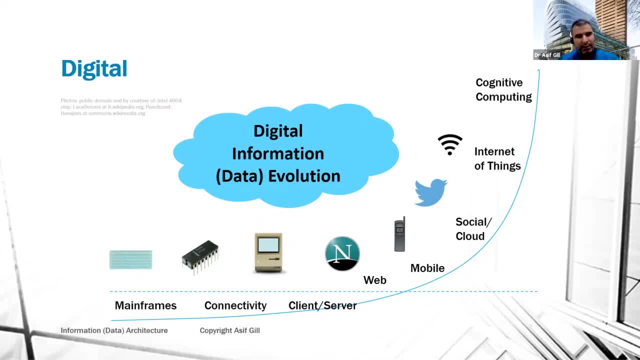 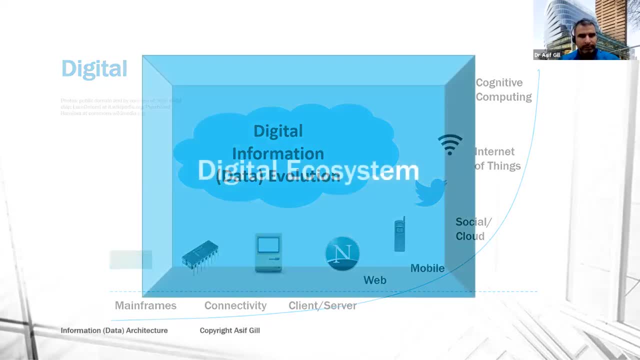 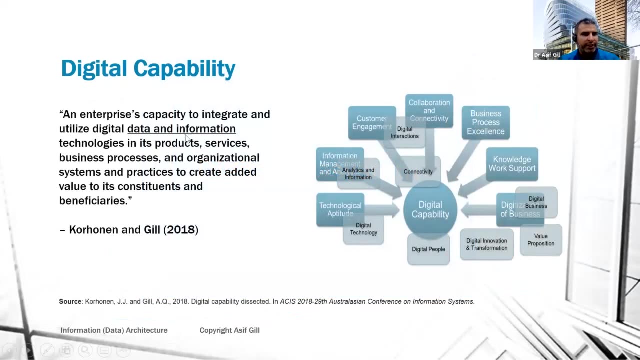 really we need to understand a holistic design or architecture of the information within our enterprise and its connectivity data outside the enterprise world as well within the ecosystem and if you look at a digital ecosystem example, it's really about the application of the technology and looking at really integrating and utilizing digital data information technologies in 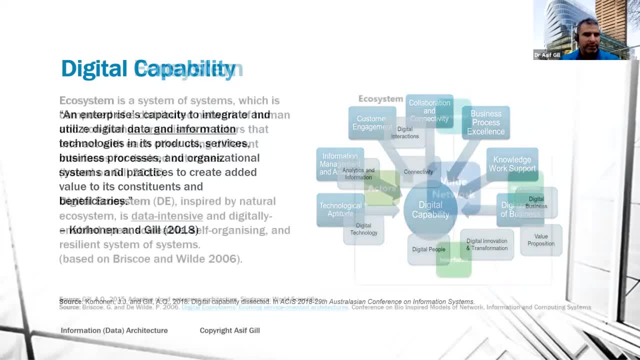 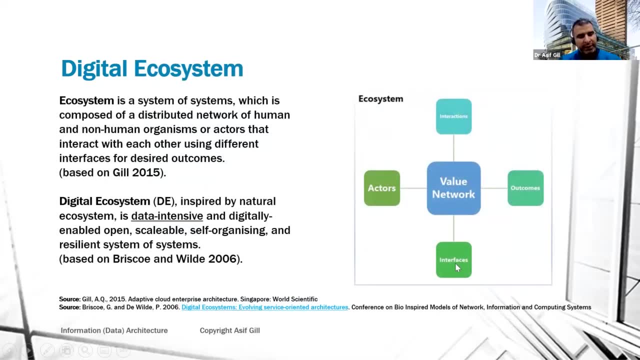 everything, including the information, and that's where we're looking in the digital capability and digital ecosystem, actually looking at the different actors. they interact with each other via different interfaces for certain outcomes. so really, when you're looking at the ecosystem view, you are actually looking at different actors and during those actors interaction, you use and 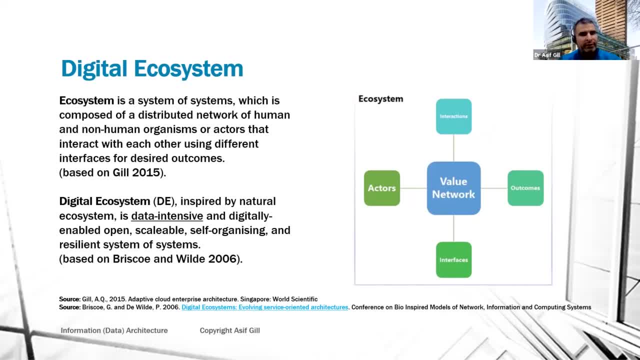 consume or produce or collect data and information and your architecture needs to be more interaction oriented architecture. we should look at the data in use and how to handle the that data and how to design the architecture of that. that's really a digital ecosystem view of the data architecture there are 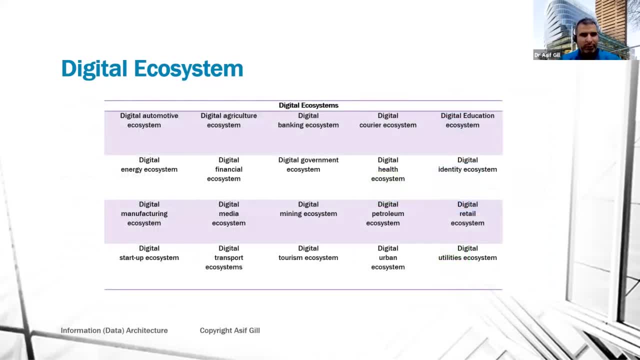 many examples of the digital ecosystem you may wondering. so we will be looking in the automobile, agriculture, banking, so different domains and they have their own digital ecosystems. it means we are looking at different domain data and those domains might be interacting as well. might be agriculture domain is. 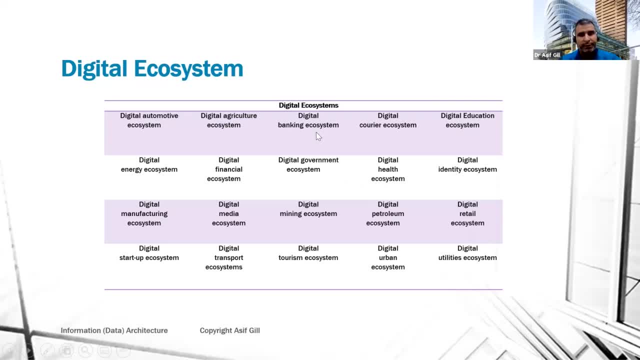 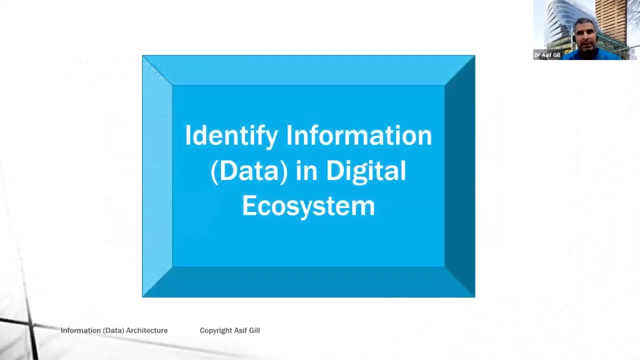 interacting with the banking domain, right from insurance purposes point of view, and other other other domain come into play as well. so we're looking at something digital ecosystem, but also interdisciplinary system as well- how the data could be shared for secondary purposes, for other purposes. so, really, data is a complex piece and we really do need to understand is. 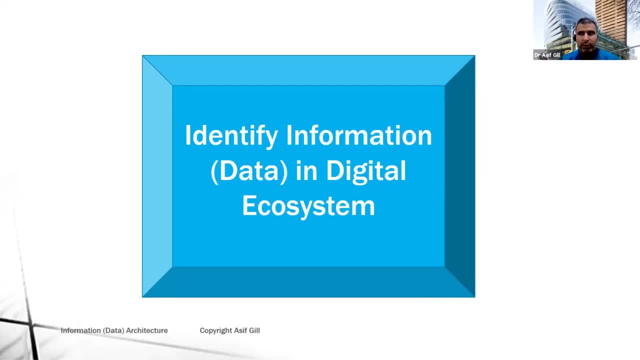 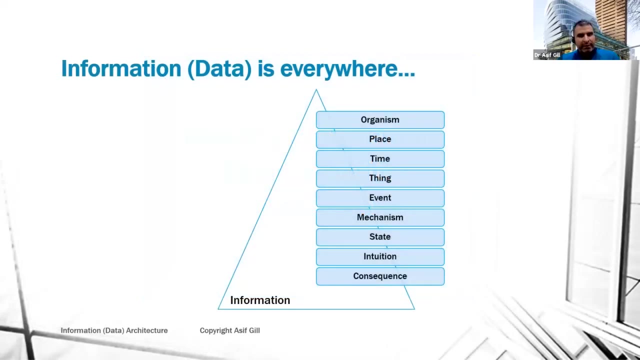 existence within our digital ecosystem. so the question is that if you are being a part of a larger ecosystem, how would you identify the data or information? so really we need some kind of a lens. information, data is everywhere. so here in the lab we have developed and user, reuse and enhance this lens where we use. 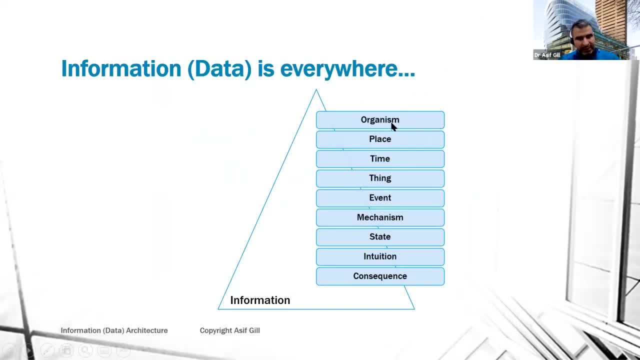 organism, organism oriented approach and organize the organisms are actors, humans, which could be known humans like organization, which are made of humans, animals, plants, all these organism which they interact with each other, they produce or produce or consume or collect data from each other and there all happens at certain place and time and they attract with certain things. so all 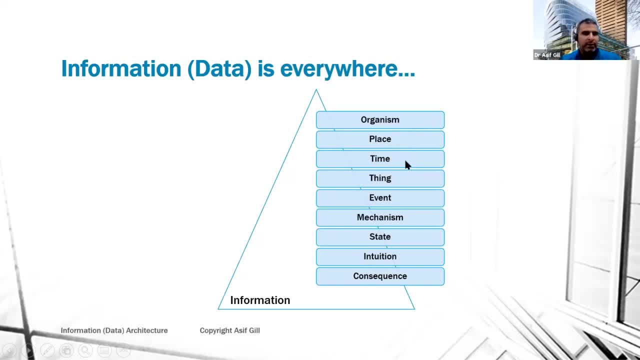 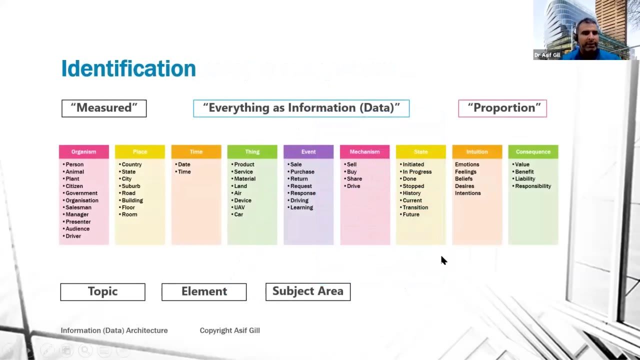 these nine items or lenses can be used to identify information which is subject to design or architecture in the future, and then we can use it to identify in your ecosystem. that's a really first step and that's an identification lens. you can see that here. I just applied here and it start from organism and from. 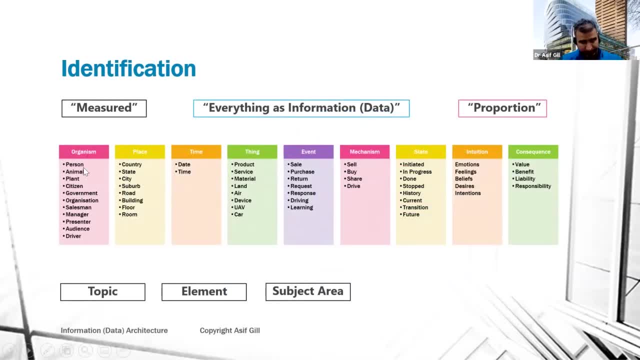 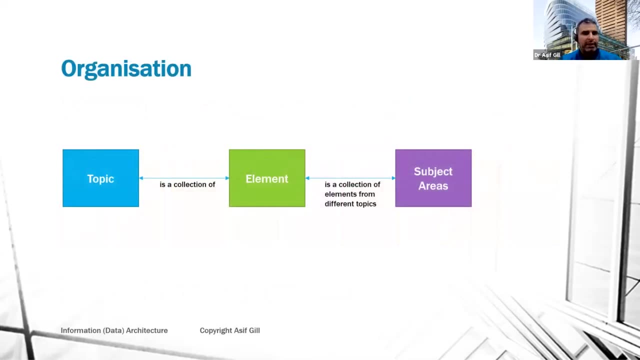 here you identify the organism in the in your ecosystem and look at that, what data the share consumer manage and that could be relevant to a place, time things and even and all these things. and once you identify the data really in your ecosystem, then you really need to organize it and that's part of the. 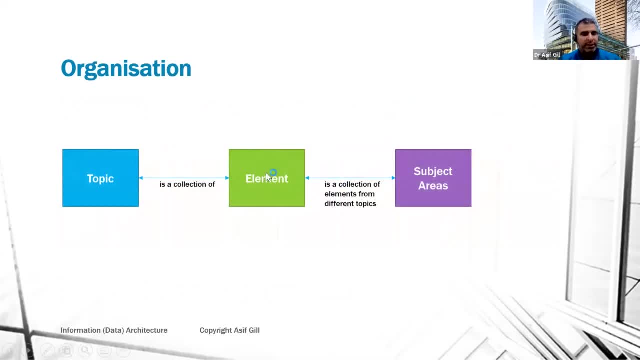 architecture as well. so an element of information identified in the enterprise could be part of a some generic topic. so topic is a collection of elements and then those elements could be included in different subject areas, so subject area can have elements from multiple topics. so really, once you identify, we really need to. 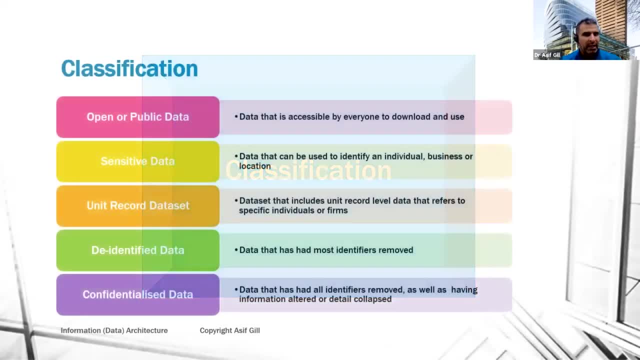 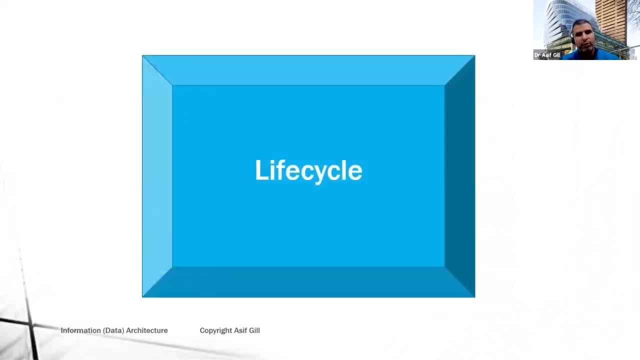 organize. once you organize that, then we need to classify: how sensitive is this data? I'm dealing with that. as soon as you identify the data, organize it and you really need to look at that- how we classify is an open data or it's very confidential or sensitive data? and then you look at- also the part of that is at: 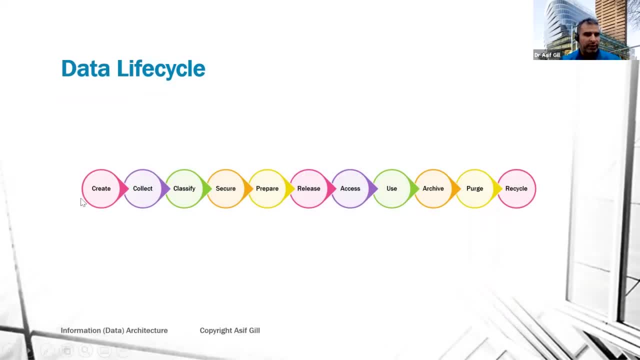 which states the data is at the moment lifecycle, so is a creation stage in all the way to purge or recycle. so data has goes through different stages and these stages are very data or information centric. you can see that here. I did not use anywhere something called storage. storage is a process or behavior. it's not. 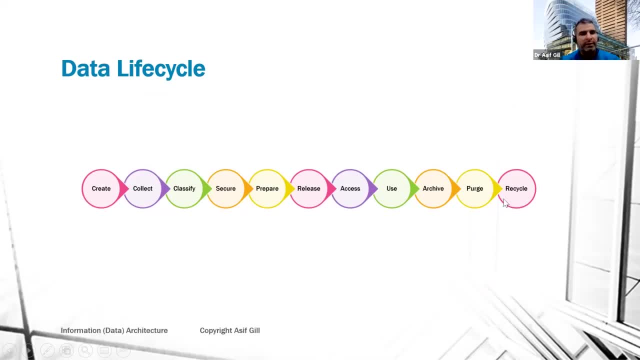 lifecycle here. I did not talk about any secondary street thing, only discuss the information element which is created, collected, classified, secure, prepare, release, access, used, archive, purge and recycle. so really you're looking at information or data element centering approach, recycle, rather than a technology century. that's really important differentiation and when you 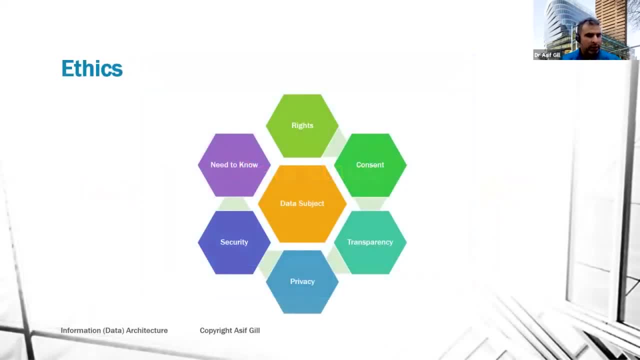 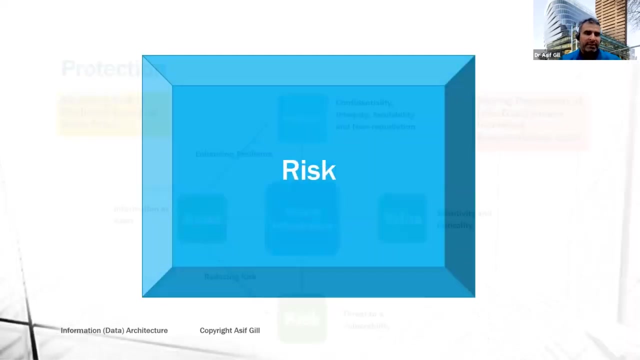 classify. you also look at that where the data used or or stored or access in an ethical manner. so really, someone needs to understand a data subject rights and there is a lot of other things around there- and also we need to look at that. what risks are attached to our information when we treat information? 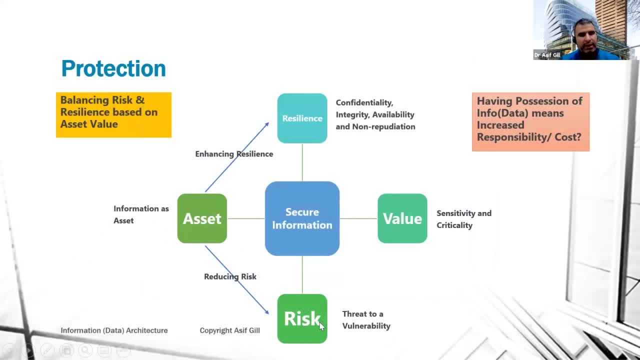 asset it's all about. and then standing your risk, reducing or minimizing risk which can be exploited by different threats, and enhancing the resilience. so really we're looking at balancing risk and resilience when we're dealing with the information, protection of your in your environment, in the ecosystem, and that's a really difficult thing. and finally, 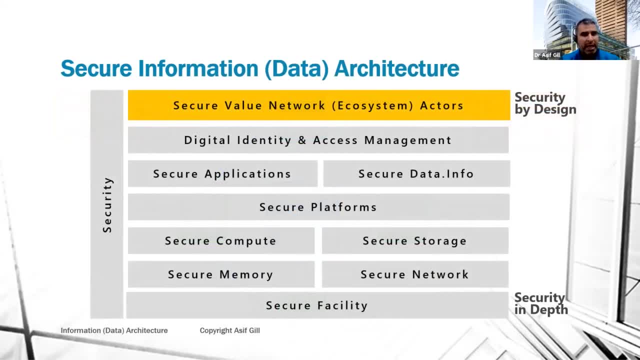 when you look at that, the protection part of is that we really actually embed your security across, or privacy or protection across, all the layers of your architecture. if I start the data interaction happening here in the value network ecosystem, we need to implement security and access there with. 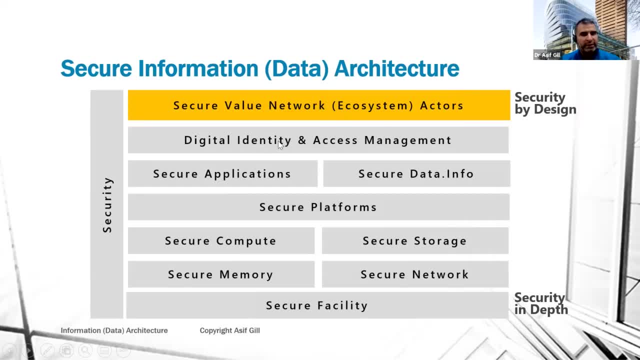 the data. also look at the identities of those actors and how they have access to your data or information, and there are information from platforms and platform having infrastructure, digital data infrastructure, and then you have the data center or facilities or physically at places where the data exists or in. 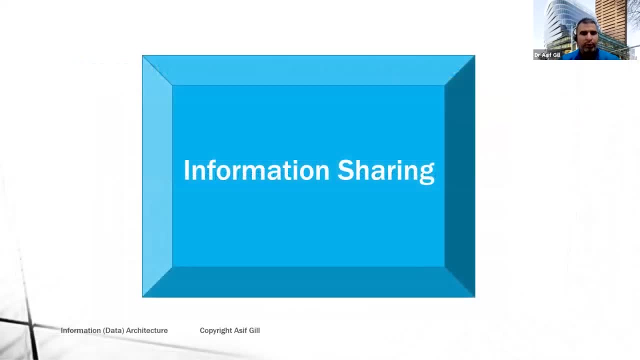 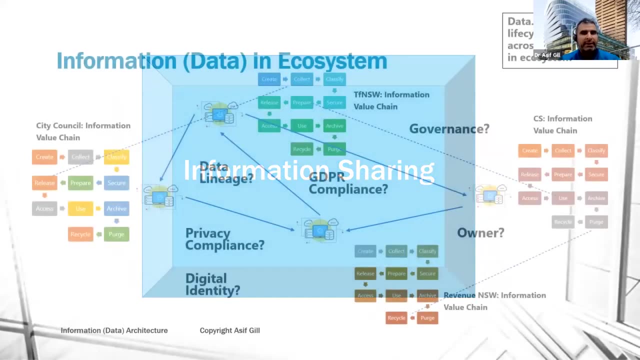 the cloud and important is that when we look at that, within the ecosystem, data is shared and that's a very really we need to understand the data, data in the ecosystem, where you can see different organizations around here. they manage the data at a different life cycle and you can see that here. let's 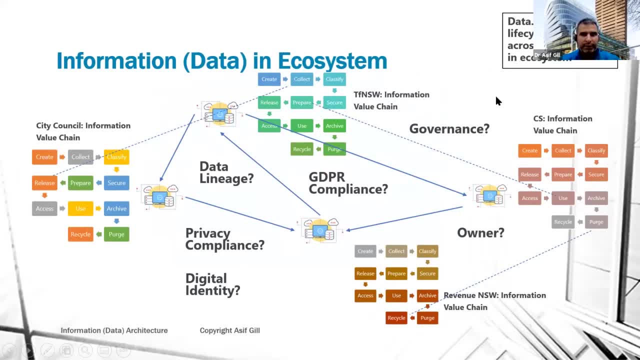 say, City Council transfer for New South Wales, customer information, customer services at your revenue start. well, they're part of a bigger ecosystem- government ecosystem- and they need to share data. but then they need to track the data lineage when data move from here to there. who owns the data when the 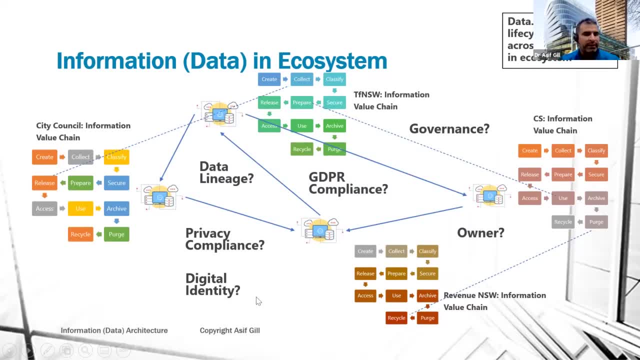 data leaves your boundary? what are the compliance and governance and privacy and digital identity or specs back. so the data architecture, information architecture, needs to deal with all these things. someone may release data here which is at the release point of the at the data lifecycle, but someone will be collecting, so data also changes its lifecycle stage as well, as soon as 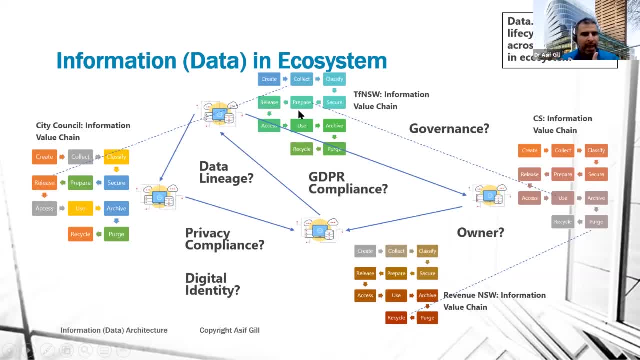 it leaves one organization to another. so how we can have a data at the multiple stage lifecycle state in different organization. how you deal with that. you can see that the data is being collected at the data lifecycle stage in different organization. how you deal with that. data architecture, information architecture. need to respond to that. 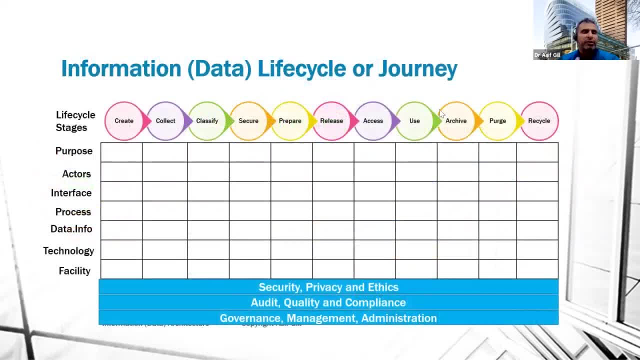 and that's where I will say that information data lifecycle journey. we need to understand in our architecture where we have the purpose around each cycle, actors involved in the data, with the each cycle interface, processes, technology facility, and we need to understand security, privacy, I think across the board, across the lifecycle of the information element, its quality. 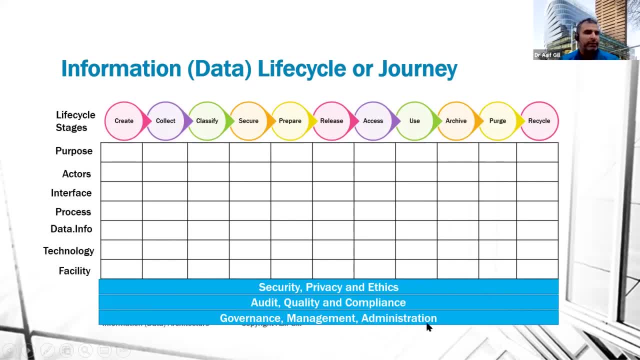 audit and compliance, its governance, management, administration of that information element. so it's really you can see that here I did not use much of a technology slangs, data breaks or cloud error or our data fabric or other thing. I just want you to focus on the information element, data elements and itself its design, because a lot of time 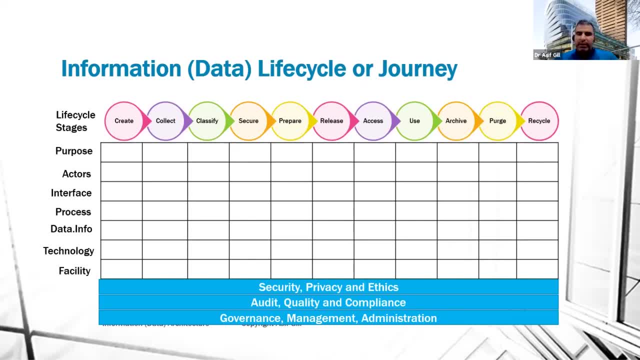 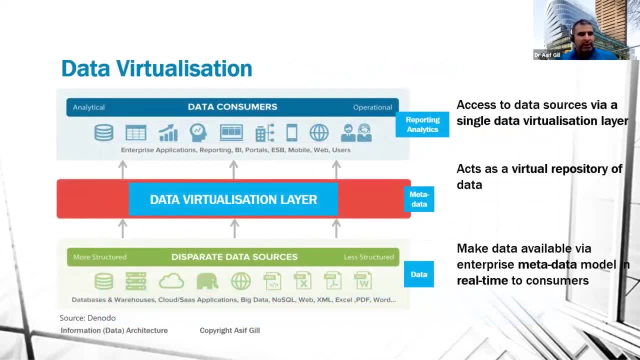 get lost in those different technology rather than looking after the data. and here is an example of the modern data architecture where we have data could be stored in different places, sources, and we need to have a data fabric or data virtualization layer design which, rather than moving the data, 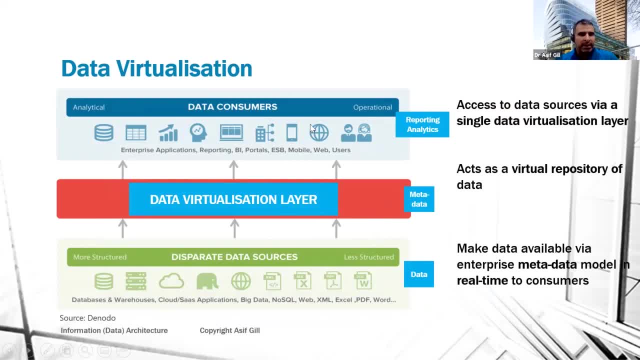 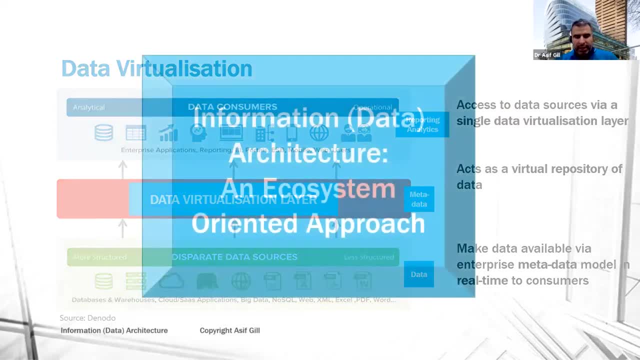 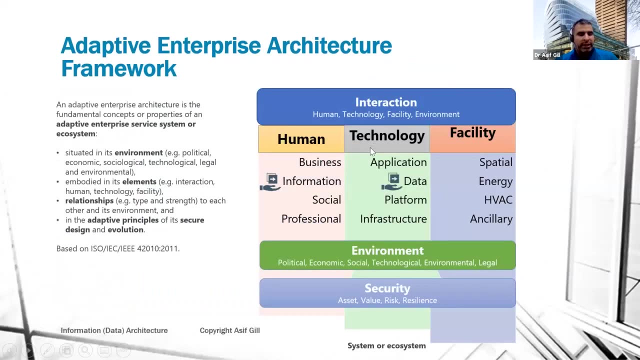 into different layers. we just allow this to accessible by sharing layer and information. data architecture and approach will, which we'll discuss in the course. we're looking at that. information is really a technology agnostic and then leads to the data and we look at the whole architecture of that from. 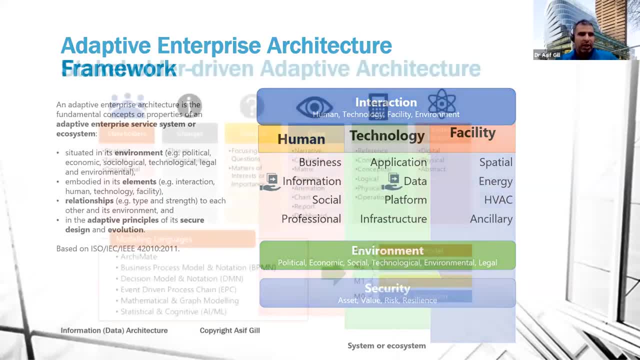 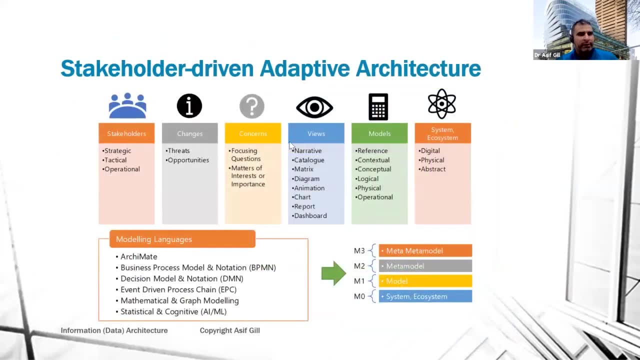 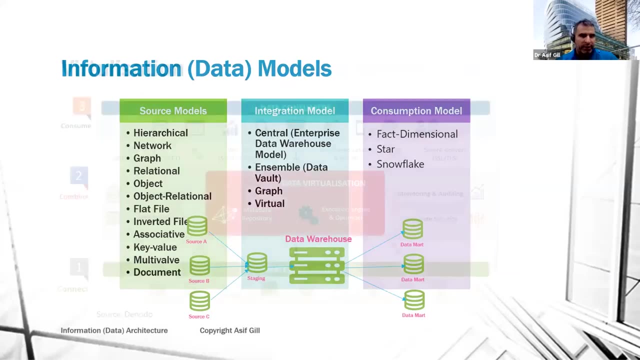 information part of you and we'll discuss in that course how we identify stakeholder concerns and how we build the information architecture using models and other things, and how we're looking at the information sourcing, integration and consumption models. and also in that course we look at that- the virtualization as well. you're also 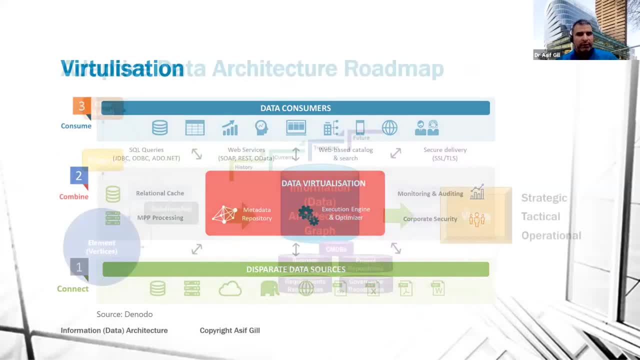 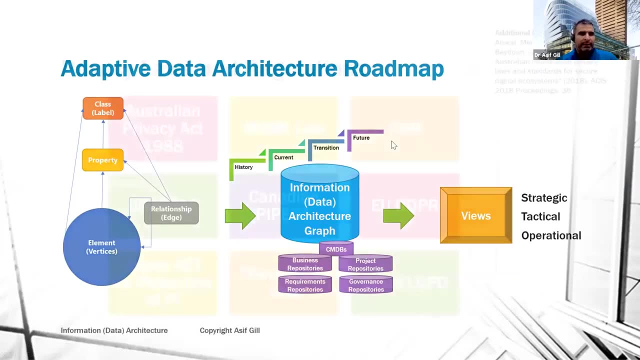 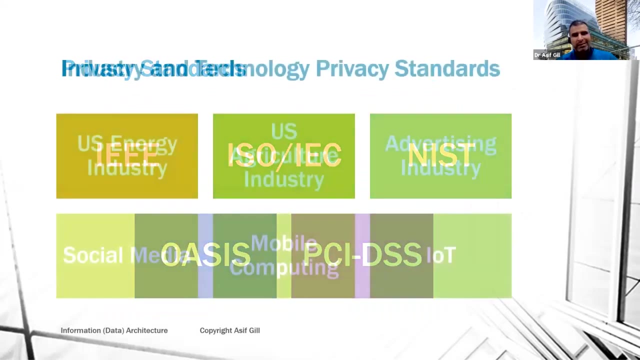 looking at the how the data architecture roadmap is developed as well for organizations based on their history, current transition and future states, and also looking at the privacy laws and regulations. in that course, we look at the privacy standards as well. impacting data. we look at the industry and 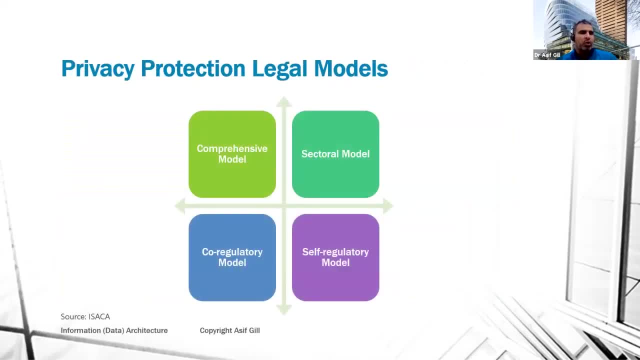 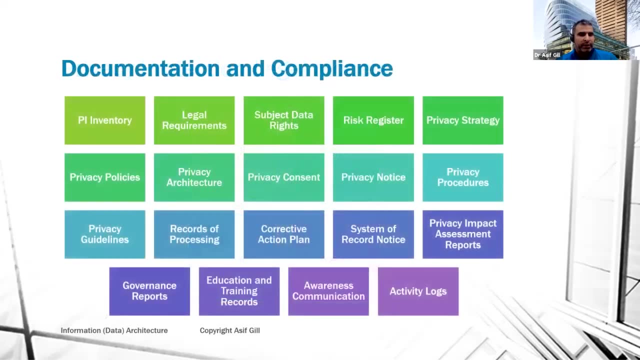 technology privacy standards as well. part of that. we look at also how the protection legal model will work for some organization. when dealing with the data, we also look at that privacy of information and what is the documentation compliance required. you can see that being a part of data. 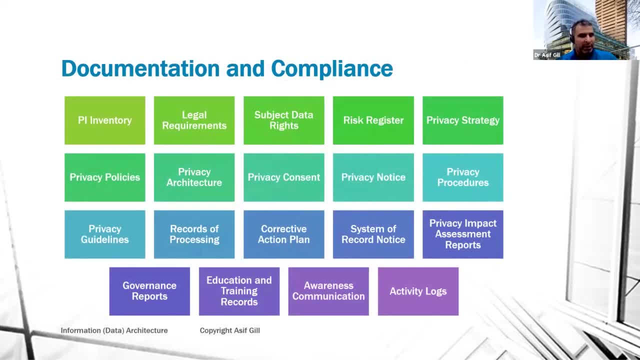 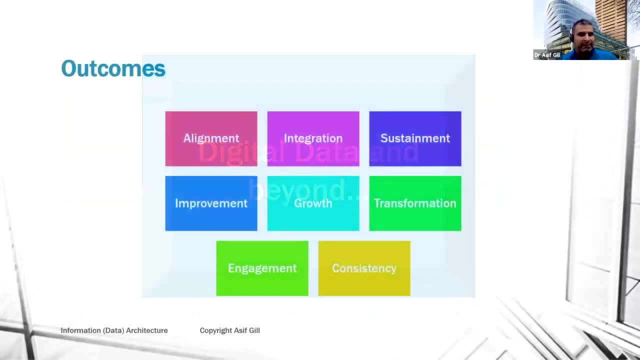 architecture is quite a challenging thing, because you need to look at, after all, the regularity and compliance requirements as well. and finally, I would say that, beyond digital data, all what we needed is that we need to have outcomes, data, information for outcome, for purpose, and that's what. it doesn't matter and when. 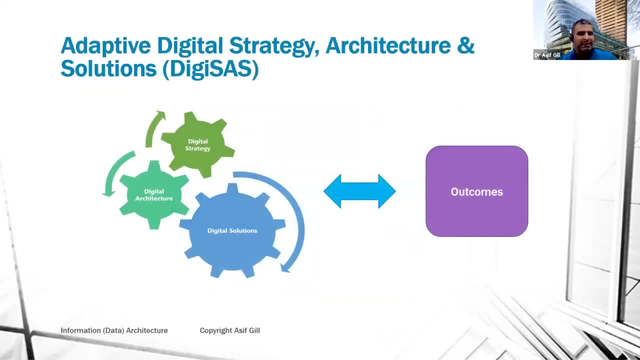 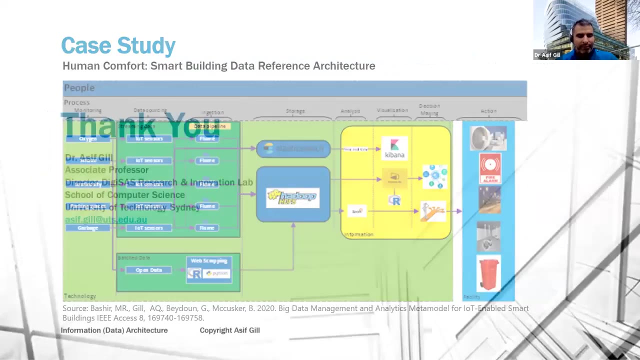 we look at the data architecture. we need to look at that across, the data architecture being a part of a digital architecture and link to the strategy and the solutions and the outcomes. and that's where I probably will stop here, the some of the case study we have done, and I think I want to just want to stop. 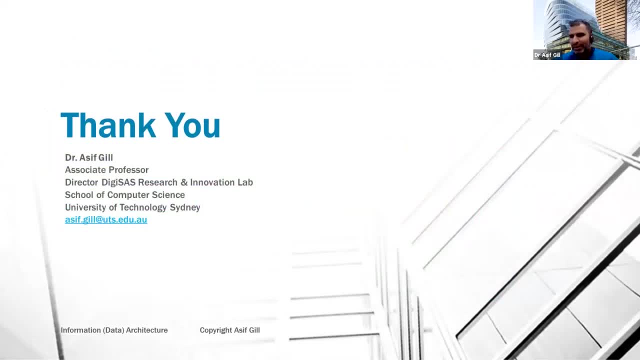 you know, I know we had a half an hour, so I'm happy to take any question. if anybody has any questions, just put them in the chat. and at the beginning you talked about you know the fact that is a shortage of information and data. architects in a struggle in Australia. I 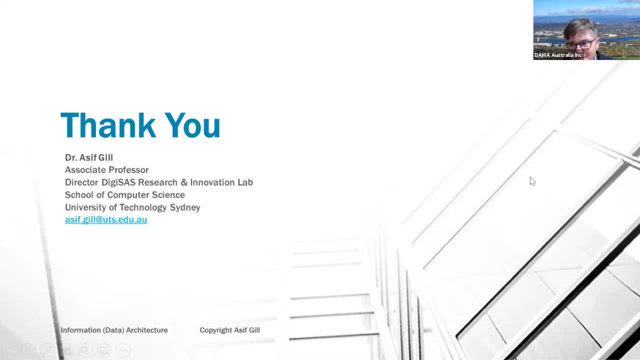 think worldwide too. so what makes a good- you know good- information and data architect? what? what makes a good one? I think I would say shifting their focus from operational development in terms of understand how to scale the performance data it is happening right now. thanks for for sharing. you know, law and order, but sugar. 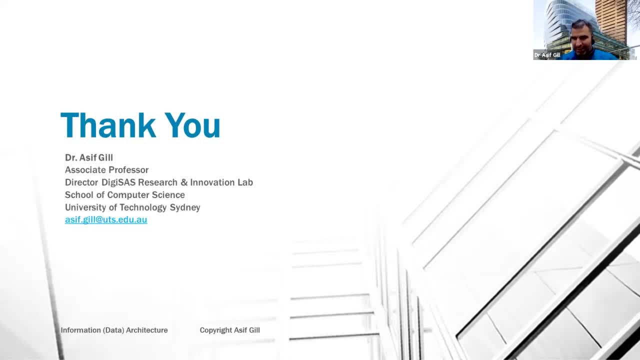 itus, more about data, students and also about policy: how to make sure our business models cropping or micro- I would say that a micro level technology view to more about understanding that business information and being able to relate to their strategy and outcomes, and that's really, really is a key piece. 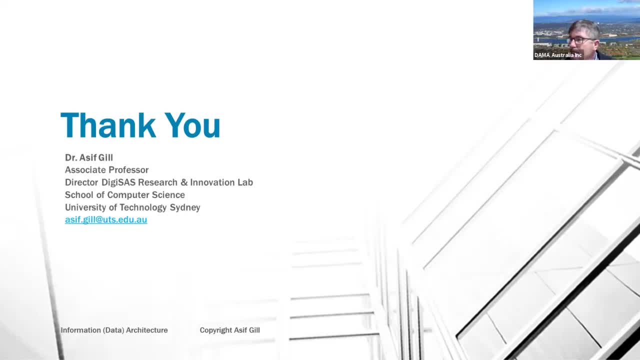 which is missing. you'll find a lot of people being able to help you with the. So what are the? if somebody's going to become an information or data architect, what are the key skills they need to learn? I think in the beginning I mentioned a lot of the areas. skills, areas identified. 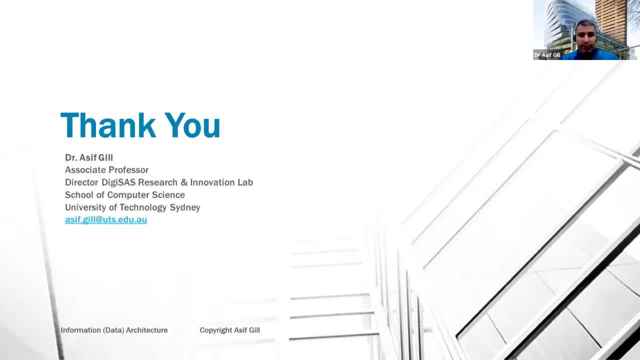 They will be able to understand and contribute to an information data strategy. They should be able to contribute or design policy. They should be able to have a good communication skills so they can communicate that policy and strategy. And also have a good stakeholder management skills, being able to when designing the stakeholder driven data architecture, information architecture which is fit for purpose and use. 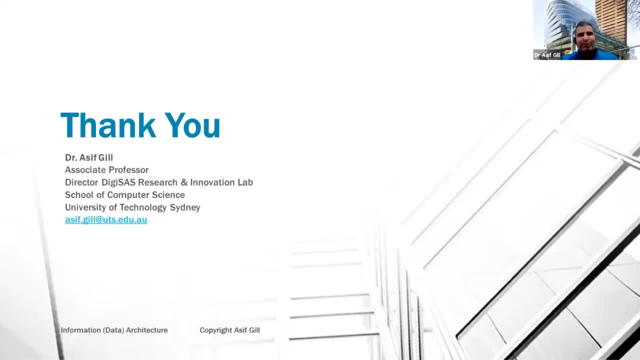 Not necessarily developing thousands of models and diagrams. That's probably is data model that can help you, But architecture need to understand that a little bit bigger picture, Right? So? So No question that comes through at the moment. So so, really this, this, George, tell us about the course, the course that you're running at Data Modeling Zone in what was it June 29th and 30th of June. 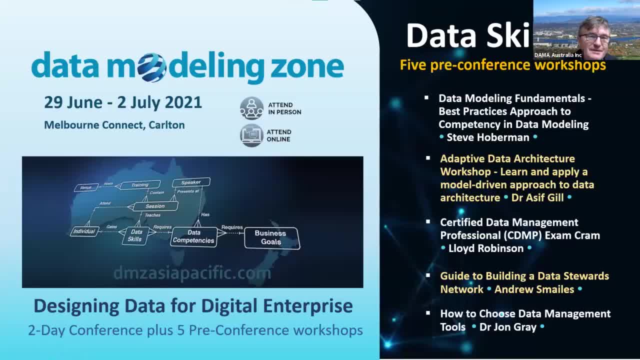 It's a two day workshop, correct, Yep. So Data Modeling Zone is a conference board of data modelers and data architects, which is an international conference is run in Australia, the US and the Europe. every year. There's a, so as if it's running. 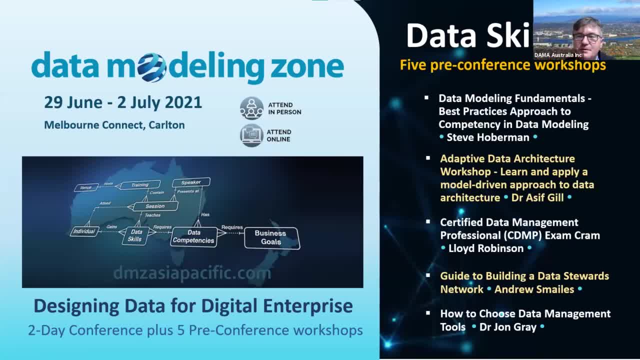 It's running a two day conference, a workshop, for the 29th and 30th of June, and then the conference itself is on the 1st and 2nd of July. So if you check out the website, all the details are there. but if you could, you would come along, as, as I was saying, there's a big skill shortage in data architecture in Australia at the moment and it'd be good to see you there. 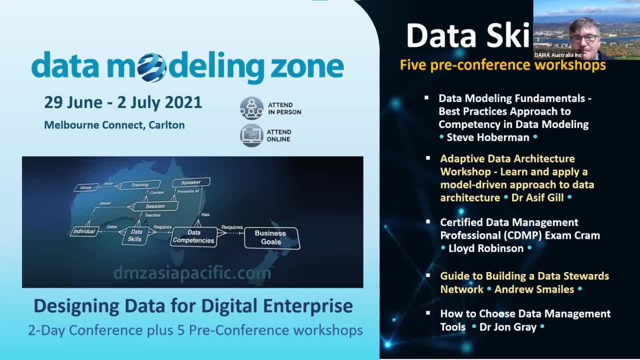 So, unless there's more questions popping up- And it hasn't been- oh, there's one. hi, this is a question. is this session recorded for members? yes, it's recorded for members and the link. I'll send out the link later today. okay, as if, can you share some of your slides too? 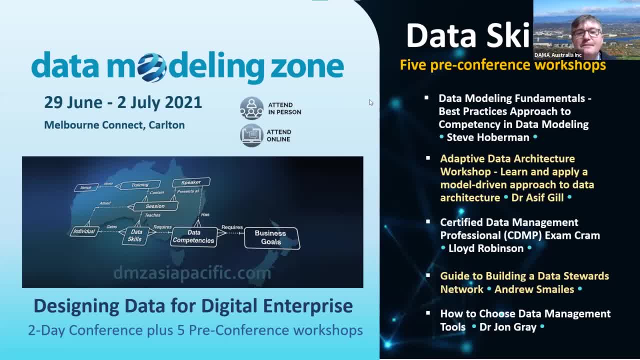 I'll be happy to. I'll be happy to share the slides. yes, Okay, all right. Well, thanks everybody. Thanks for joining, Thanks for joining the webinar. I think that was very informative and I hope lots of people watch this. 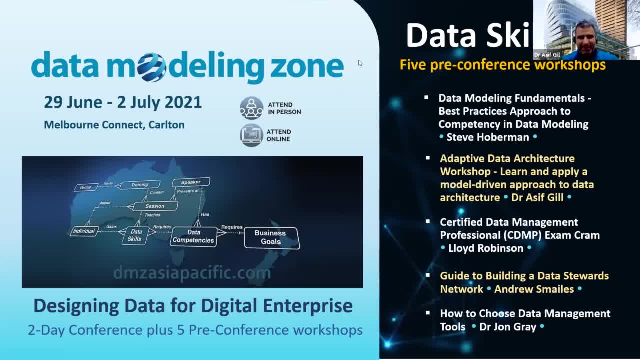 Thank you very much. They need to learn anyway. yeah, Absolutely. Thank you very much. Thanks everyone. Thanks, Andrew Bye.